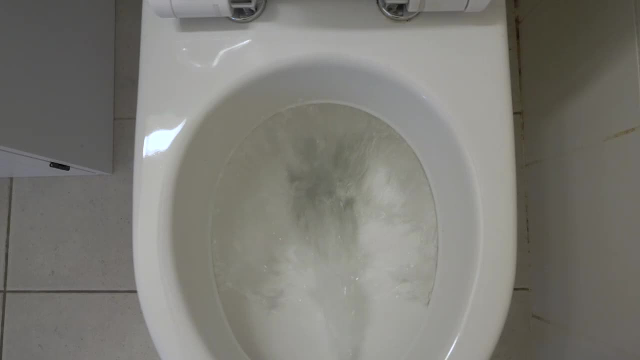 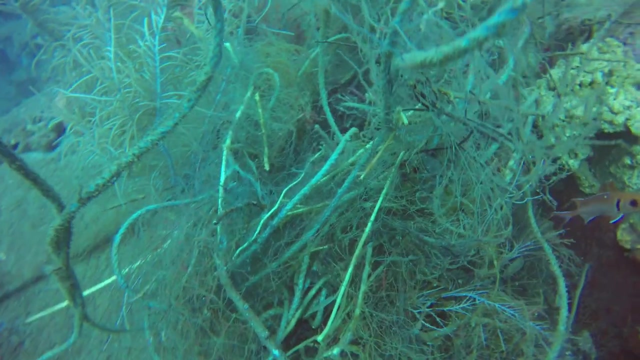 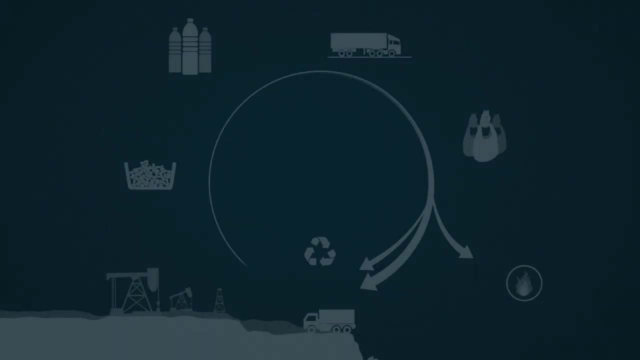 during the lifespan of plastic products. Sewage systems, rivers and discarded items at sea, such as ghost nets, are some of the ways plastic enters our oceans. Every day around the world, we use millions of single-use plastics. We need to shift from. 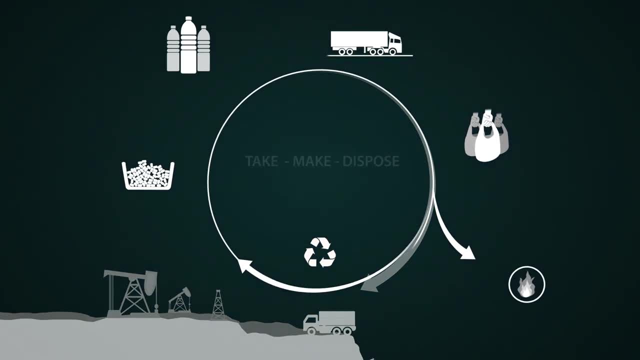 today's linear take-make-dispose model to a more circular economy in plastics' value chain, where products are designed to be used for a greater purpose. Plastic pollution is caused by the growing number of plastic waste in the world. Plastic pollution is caused by the growing number of plastic waste in the world. Plastic pollution is caused by the. 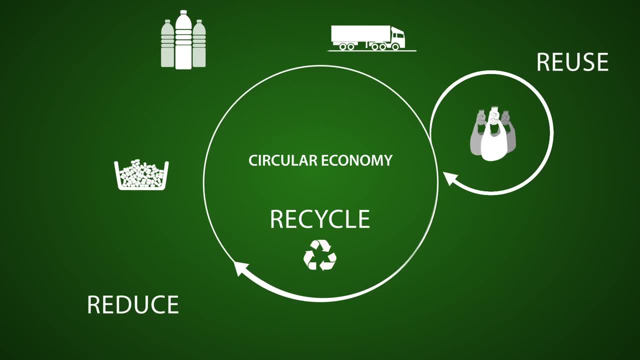